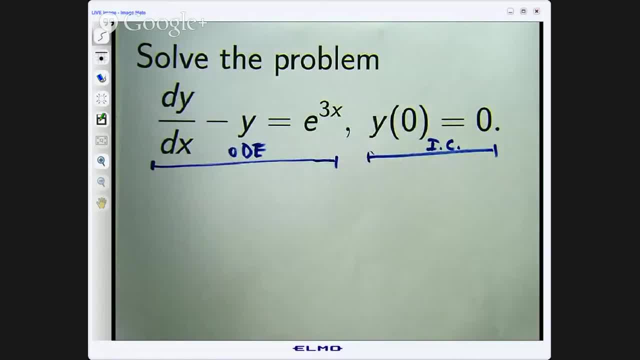 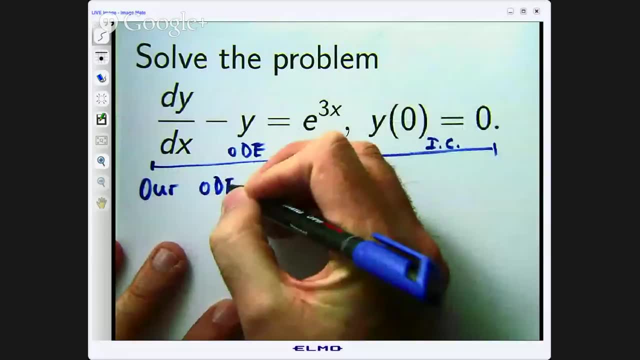 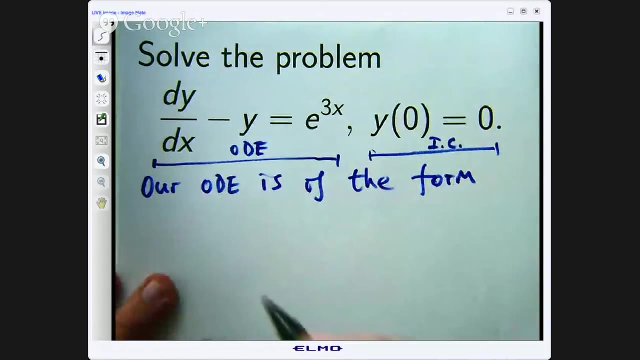 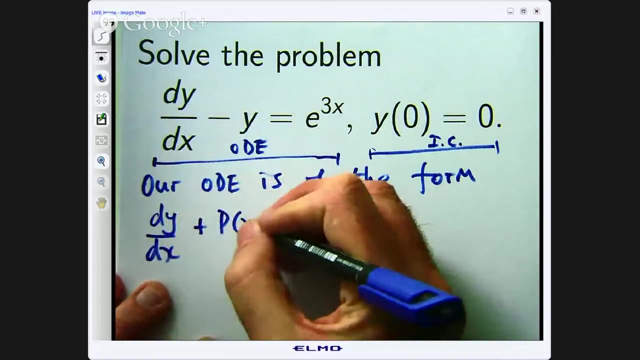 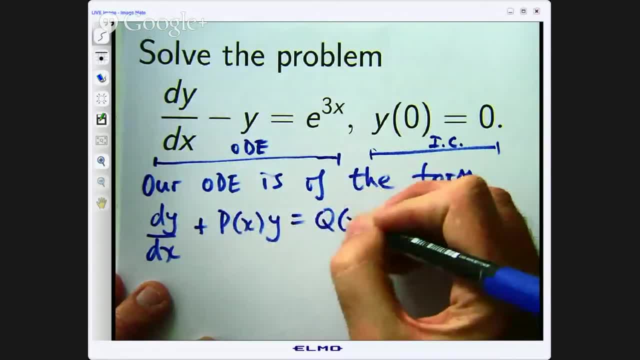 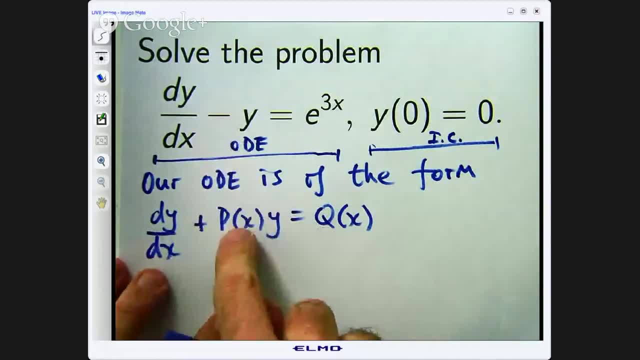 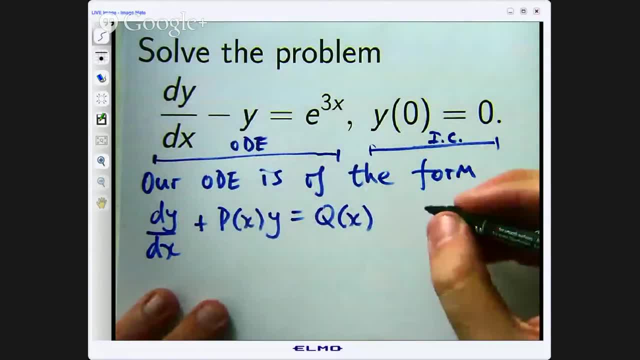 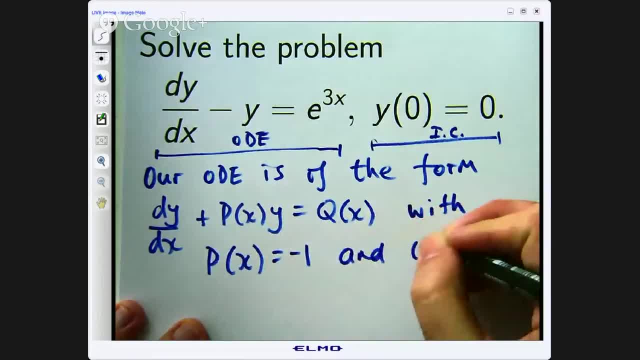 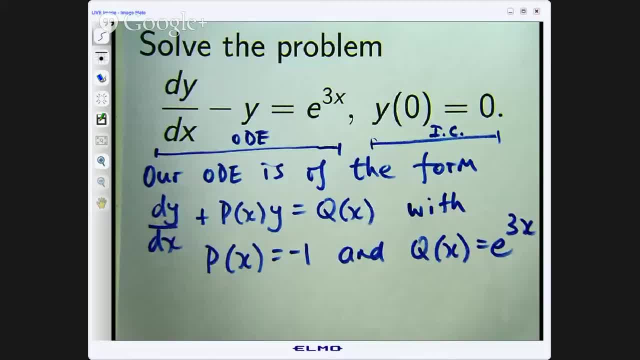 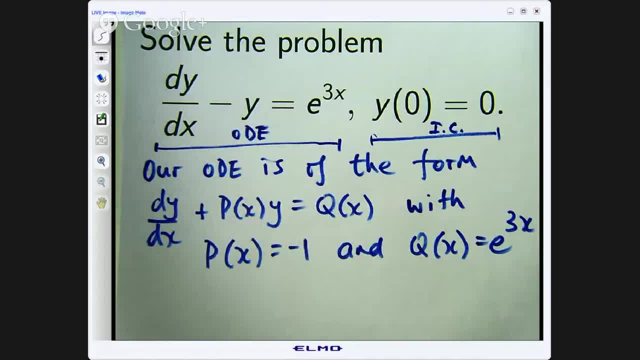 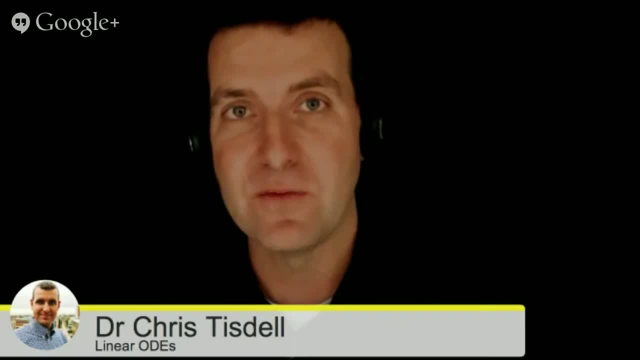 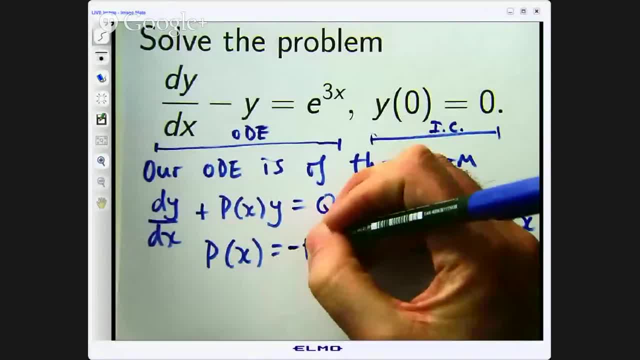 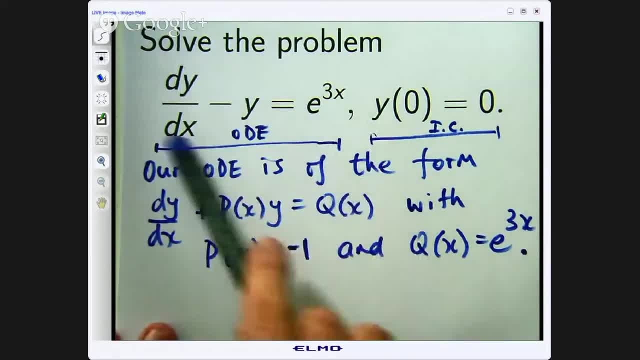 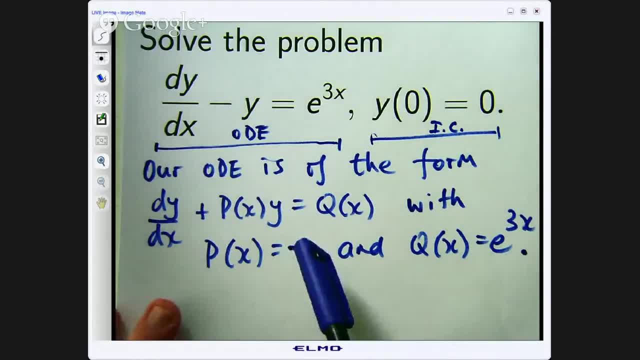 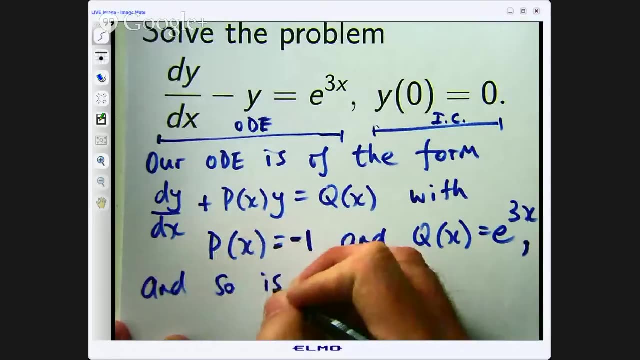 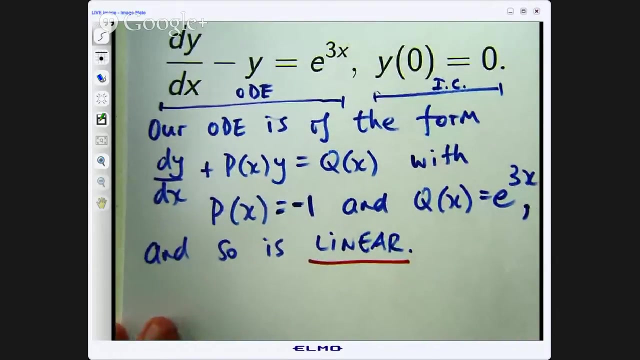 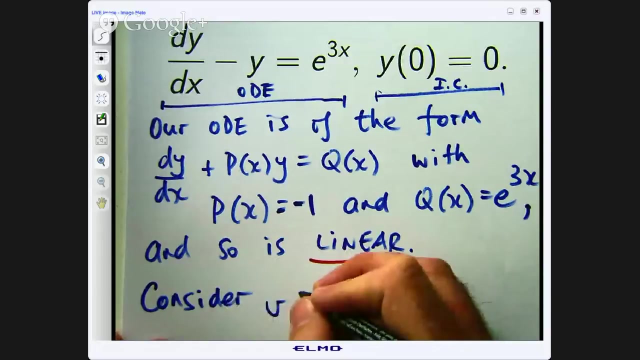 dy dx plus p x, dy dx plus p x, And you come up with the integrating factor through the coefficient function of y – the p. Alright, so let us just write down our conclusion. Okay, so Let us consider the following: I am going to introduce a function v, which is going to be this magic function. 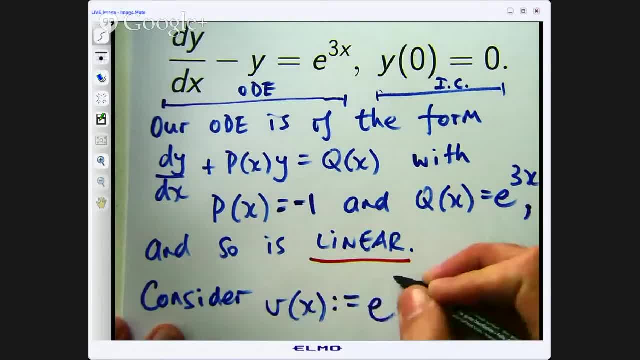 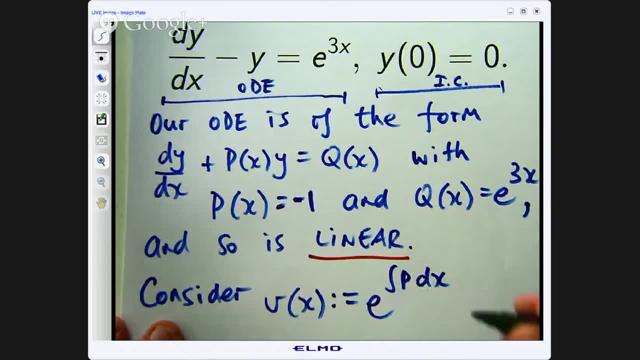 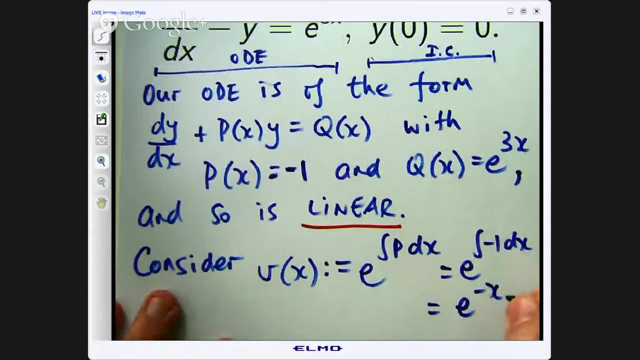 the integrating factor and it is going to be e to the integral p dx. Now you might want to put p there. I have just put p to save a bit of space. So our p the coefficient is negative 1.. So if I integrate this I will get e to the negative x. Now I do not need 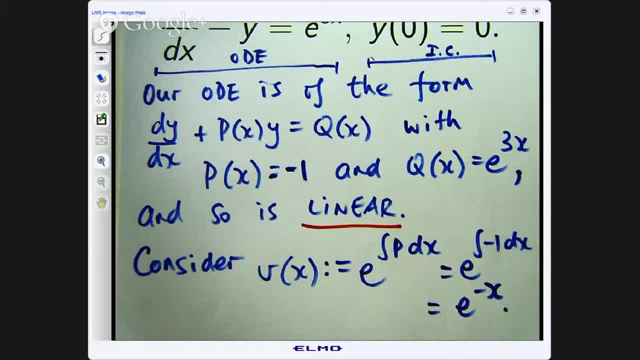 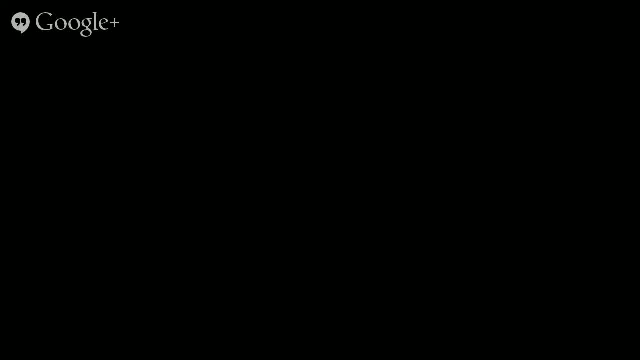 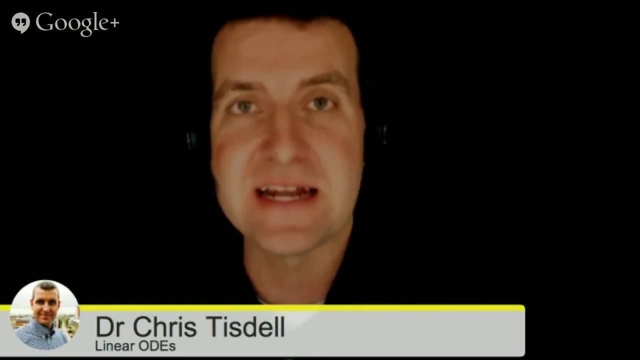 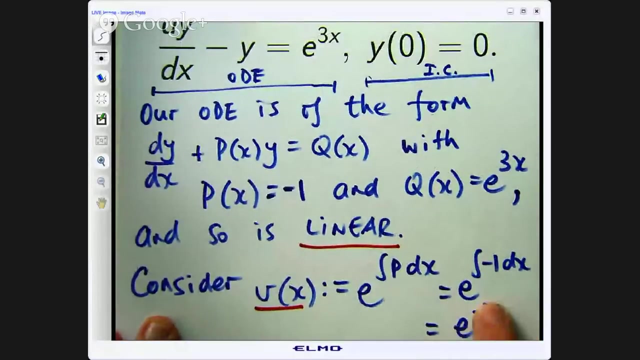 a constant of integration there. if you really feel strongly about it, you can put one in. So what we are going to do with this magic function is multiply both sides of our original differential equation By that magic function, that integrating factor. So let us do that, Let us take this e to the 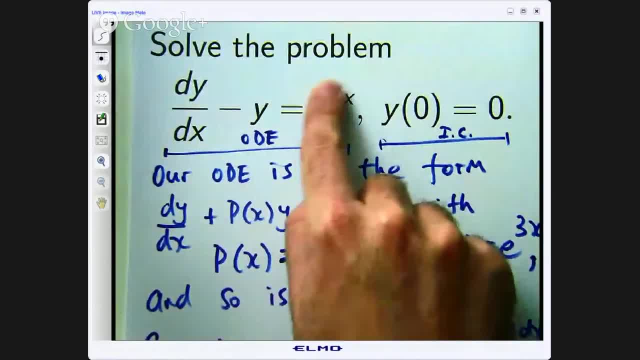 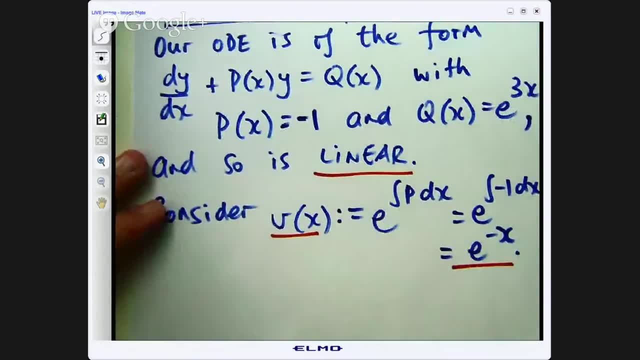 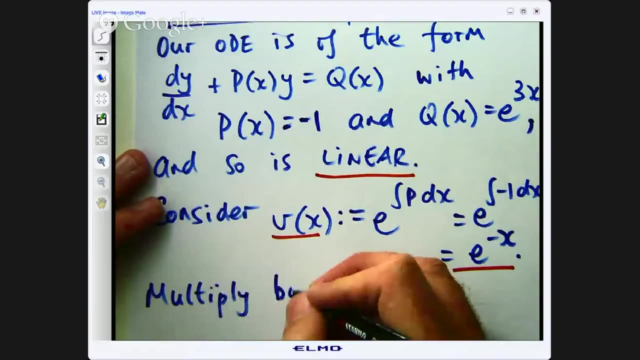 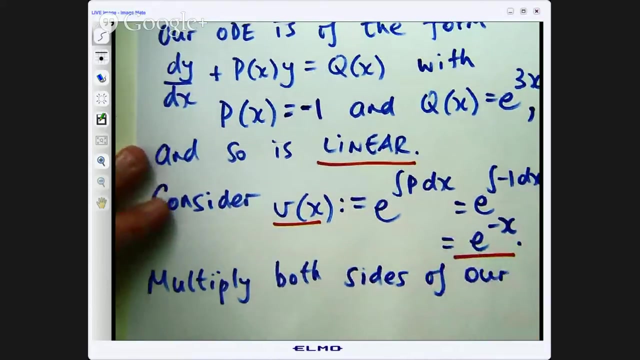 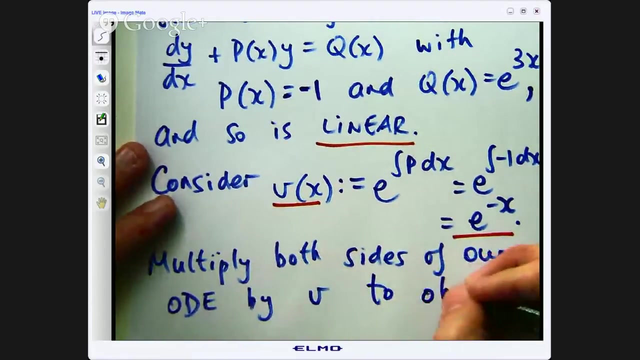 negative x and multiply both sides over here and over here by e to the negative x. Now the good question is: why would you want to do that? Well, it will become clear in a minute. So multiply both sides of our ODE by v to obtain the following: Now, v equals e to the negative. 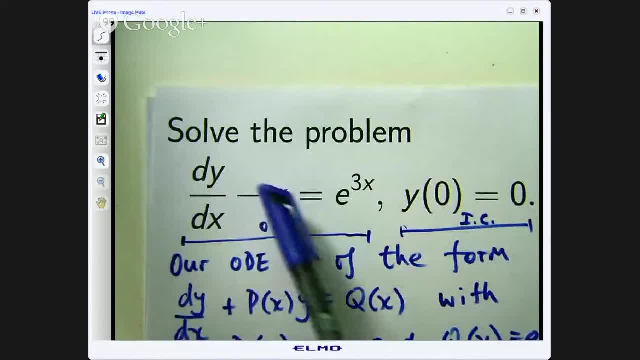 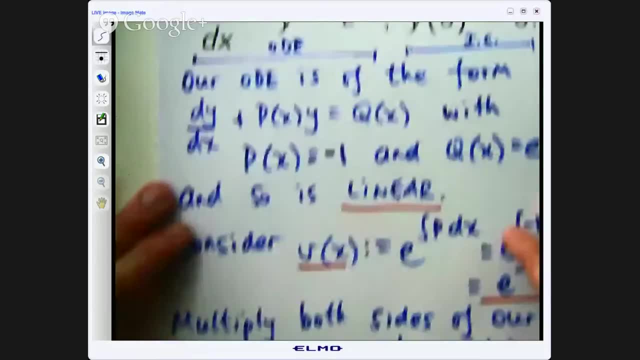 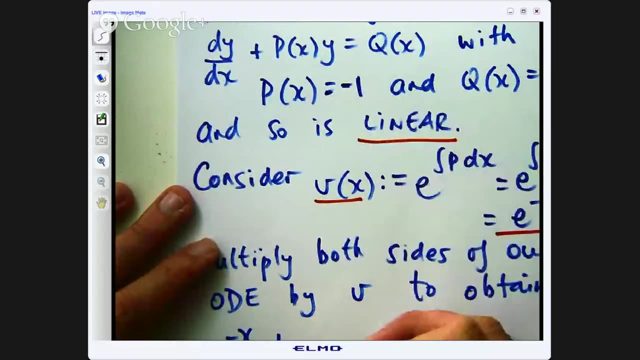 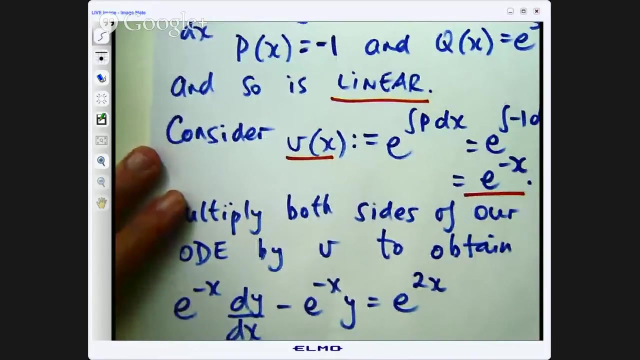 x. So I am going to get e to the negative x here, minus e to the negative x there, and multiply this by e to the negative x will give us e to the 2x. Okay, So I am going to get e to the negative x大丈夫. 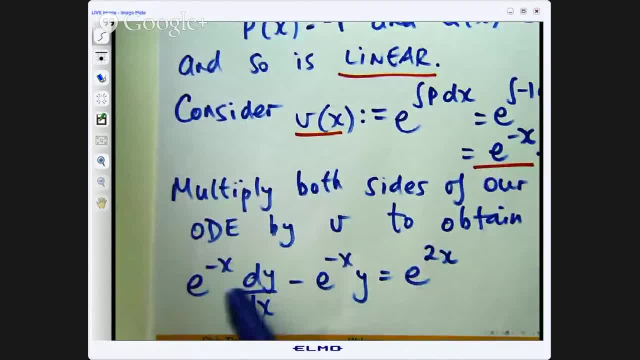 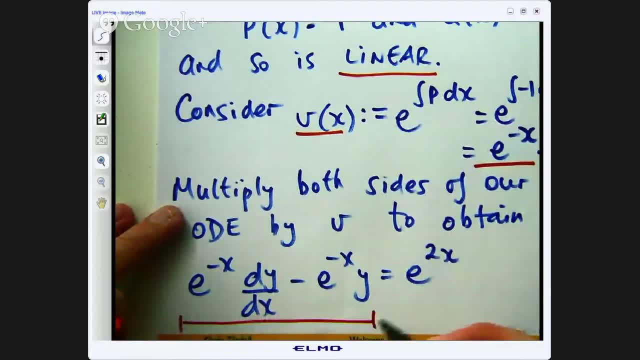 Now you might thing, experiment what I am going to do to get myüm here. Well, I'm going to do in the second part, The second part. I will run one over. look, this is where the anglophone goes. All right, all right. So now you might think: well, hang on, this website looks very messy indeed. What is going on here? Well, what is going on here? This technique allows us, by multiplying through, by this: 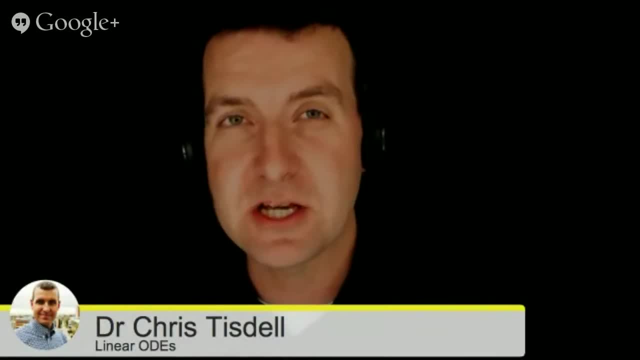 magic function, this integrating factor. it allows us to compress the left hand side down to the derivative of a special product. Okay, let me say this together: that again, the left hand side of the bottom line is going to be compressed to the derivative. 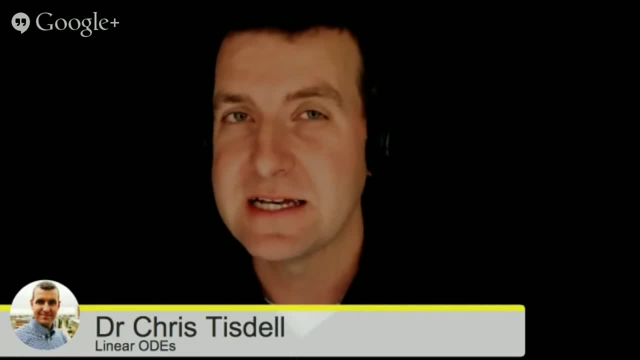 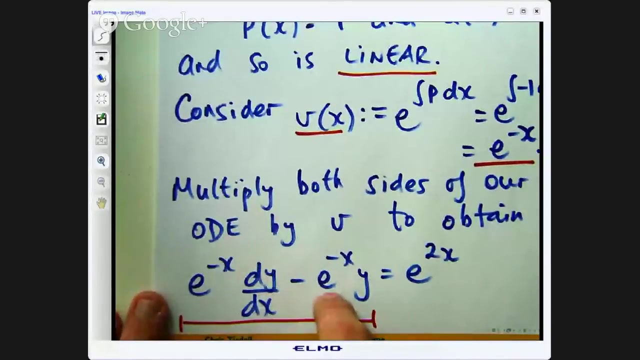 of a special product. Now that special product is going to include the unknown function y and the magic function, the integrating factor, that in this case e to the negative x. So let me share that with you. Now, if you look closely at this, this is actually the derivative. 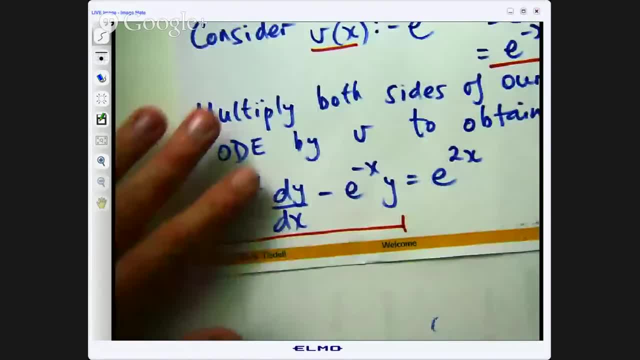 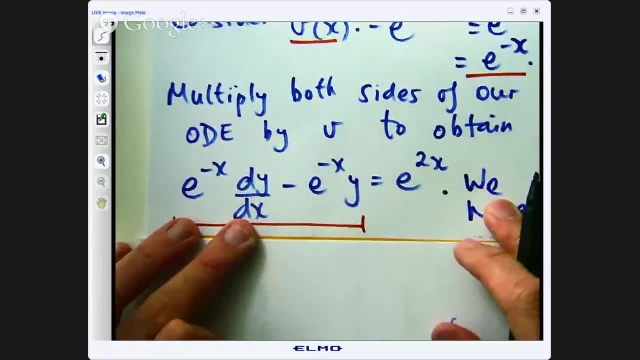 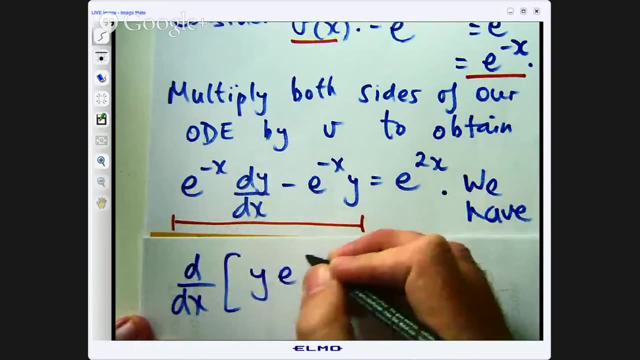 of the special product that I was telling you about just before. So we have the following: Left hand side is the derivative of this. Now you might go. well, hang on, how did you go from here to here? Well, actually, you can kind of work backwards here. 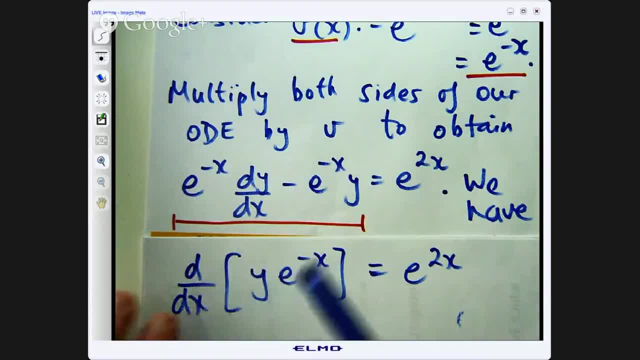 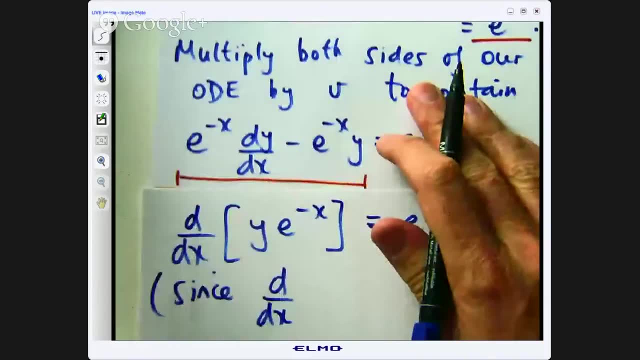 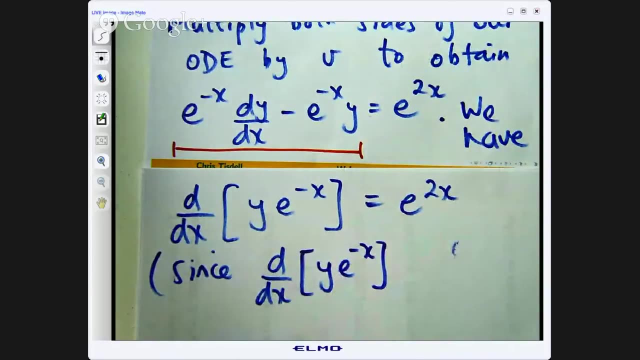 So if y is a function of x and you differentiate this by the product rule, we are going to get this left hand side. So let me just sort of justify this to you quickly. It is a product rule, so it is d? dx of y times e to the x, plus d? dx of e to the negative x times y. So this: 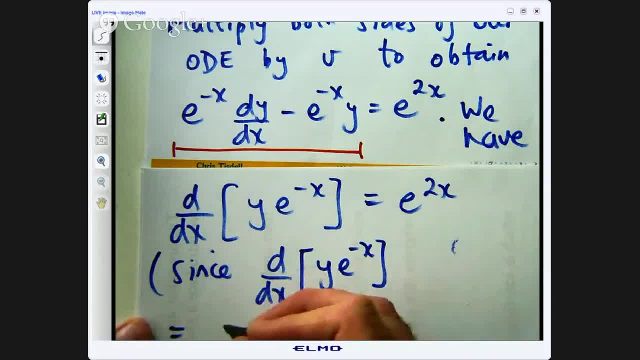 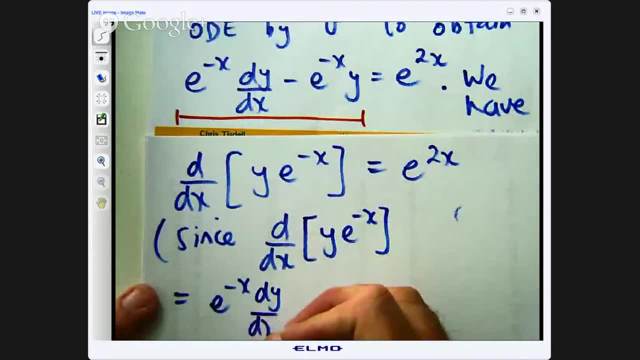 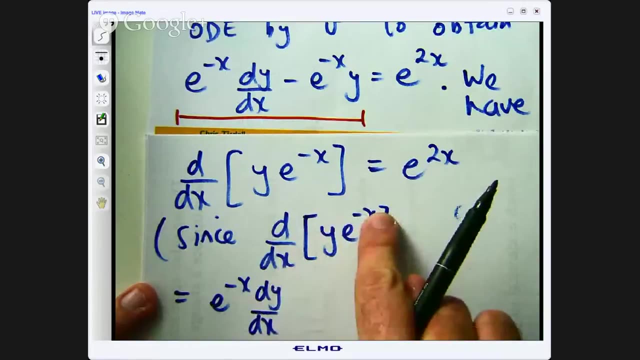 is going to be a direct function, So it is yep, d dx of y, where we don't know what y is, but it is just dy dx plus y times d? dx of e to the negative x. okay, d? dx of e to the negative x. the negative 1 comes. 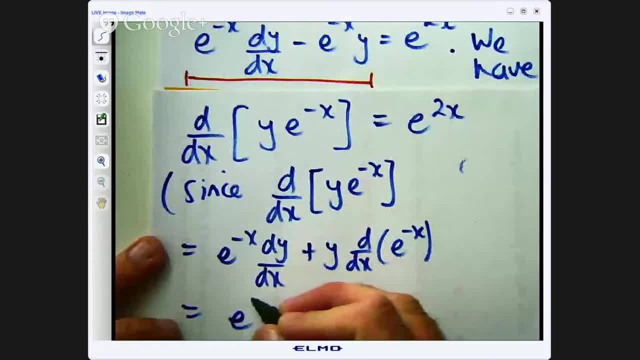 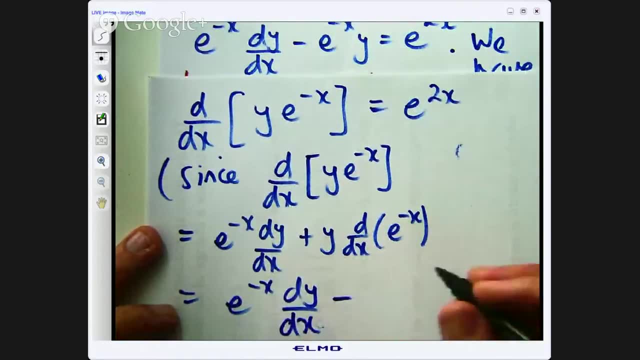 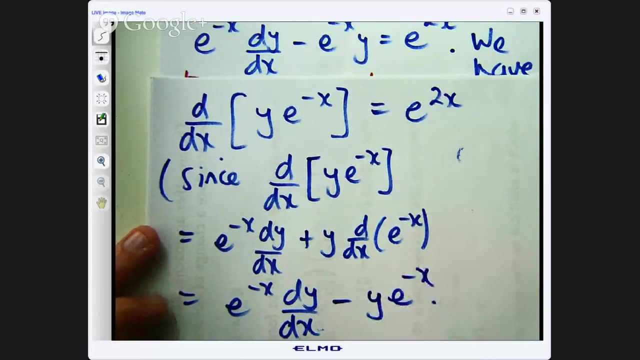 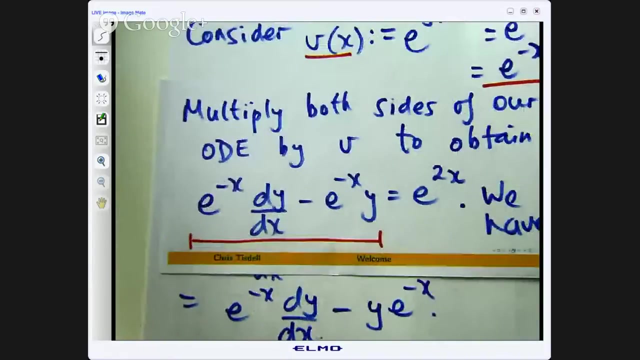 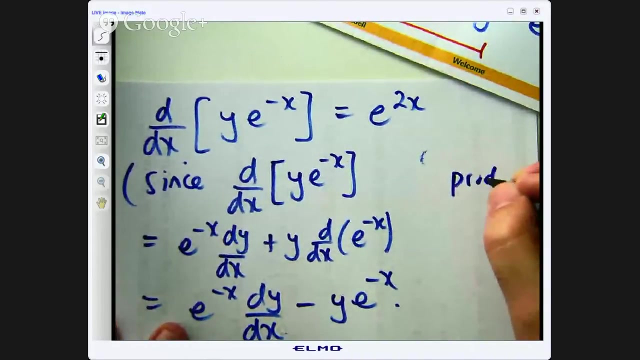 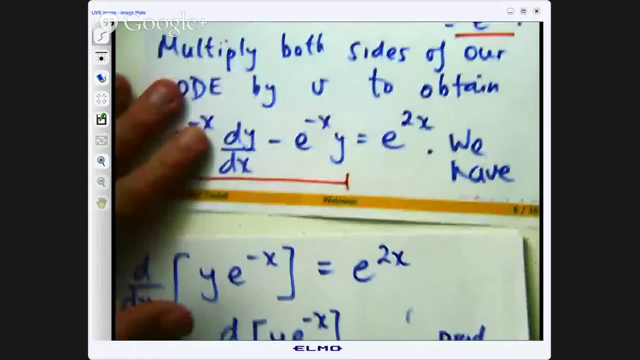 to the front. Okay, So that will be a – okay, now, this and this are exactly the same. okay, that is just switched around, alright. So what I have tried to – here I have been using the product rule, differentiation, alright. So another important thing here is: whatever the integrating factor is for different problems. 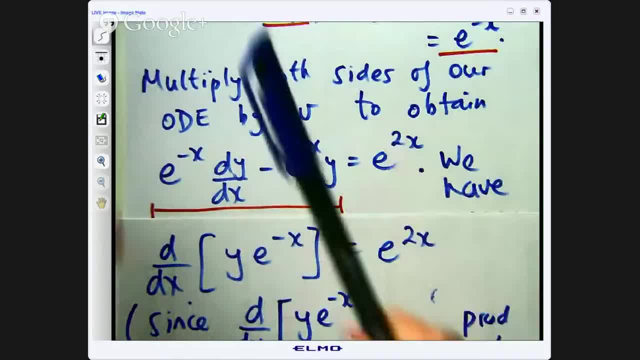 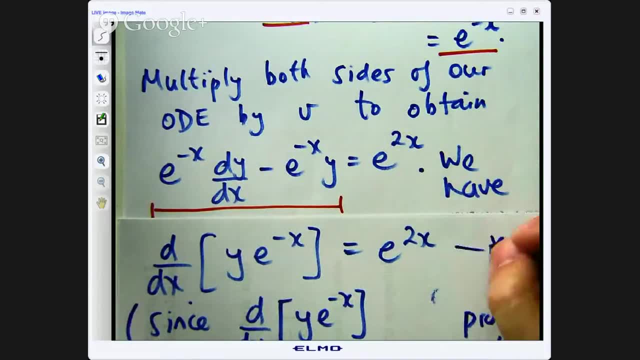 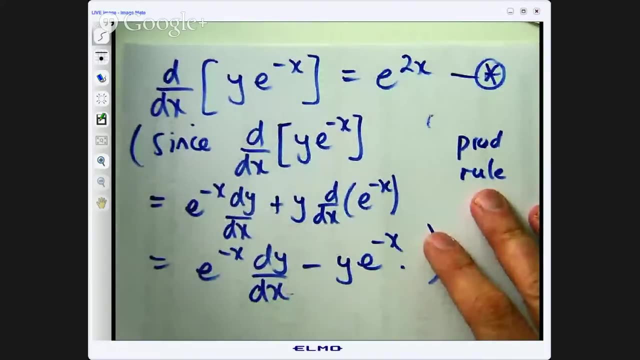 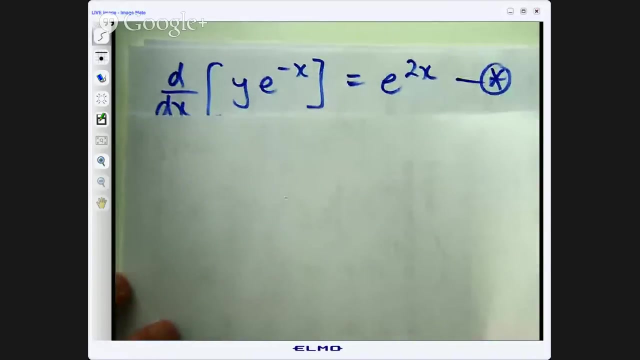 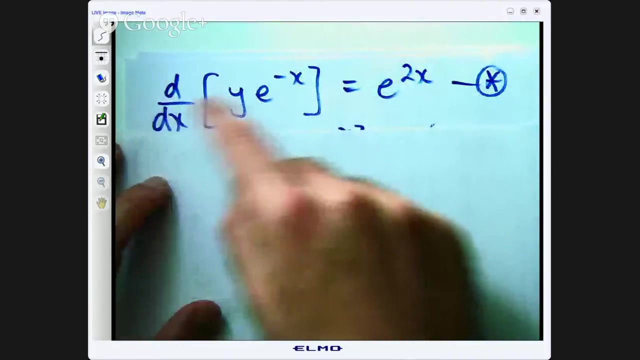 you will always get this left hand side will always compress to the derivative of the unknown function y times, v, whatever v is okay. So let us move on from star then. Okay, let me start a new page, alright. So what can I do now? well, I have got the derivative of the unknown function times that I can integrate. 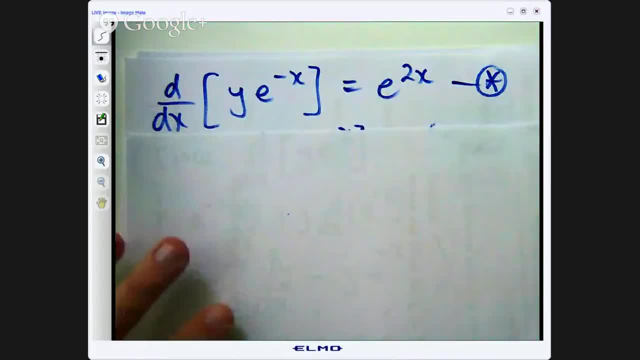 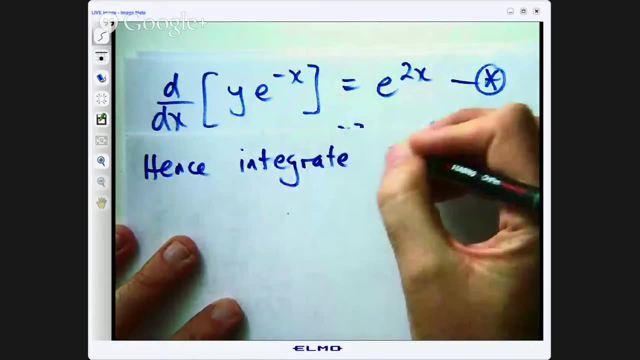 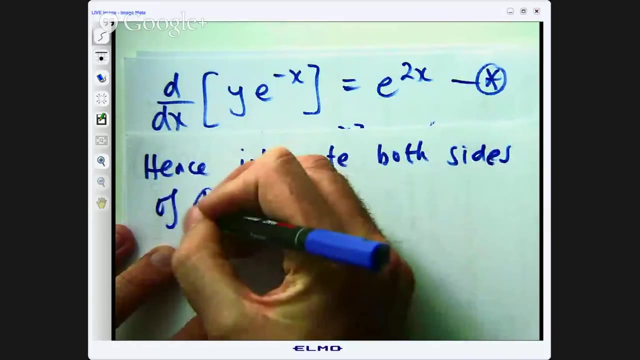 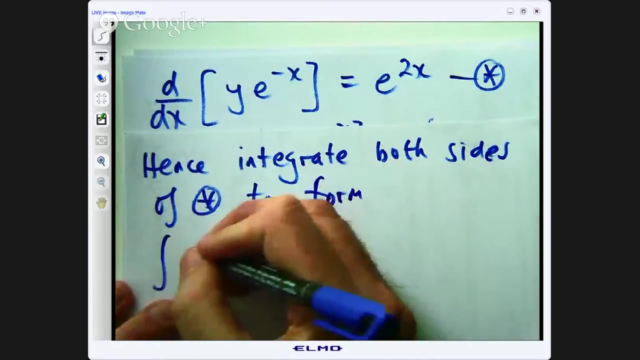 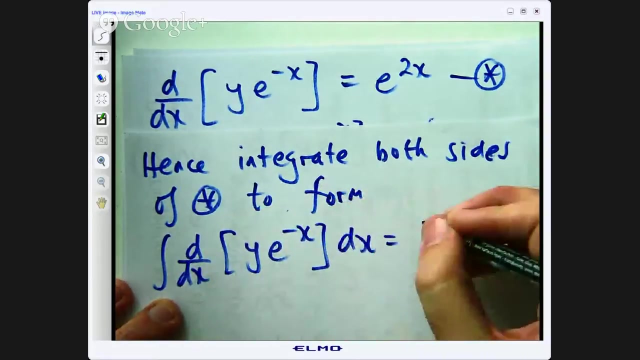 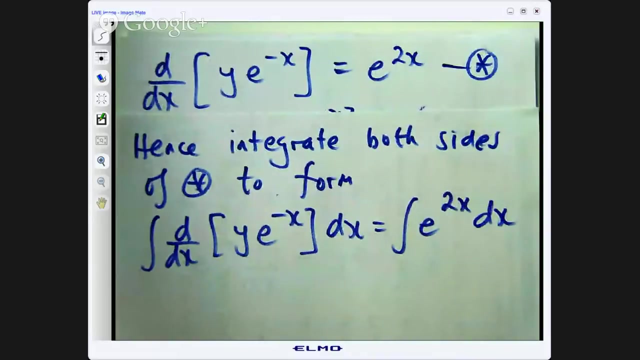 both sides and I can get that y out. okay, So we are going to integrate Both sides of star with respect to x to form the following: yeah, Now we know integration and differentiation are the opposites of each other, so that will disappear. When I integrate this, I will get e to the 2x times one half and I will put a constant. 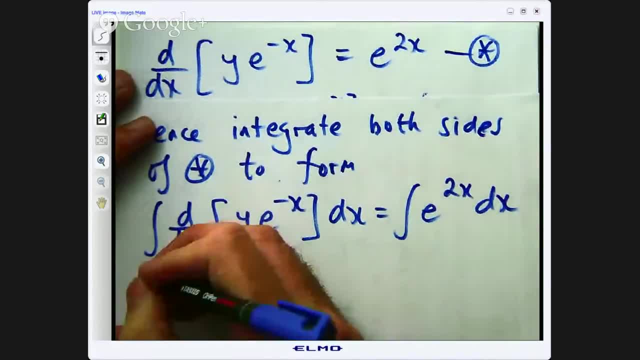 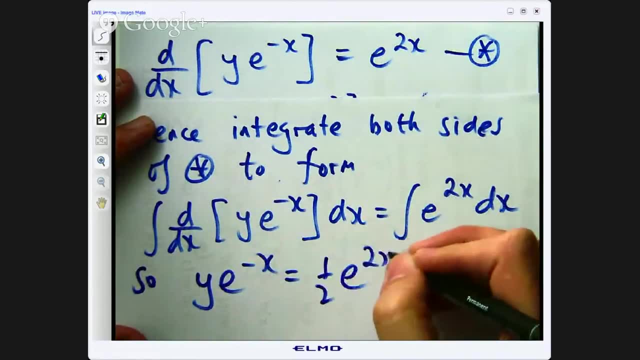 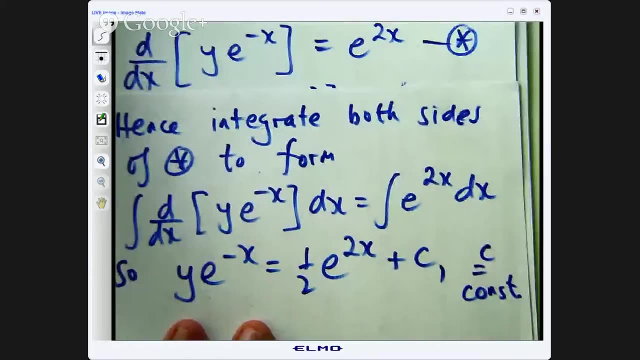 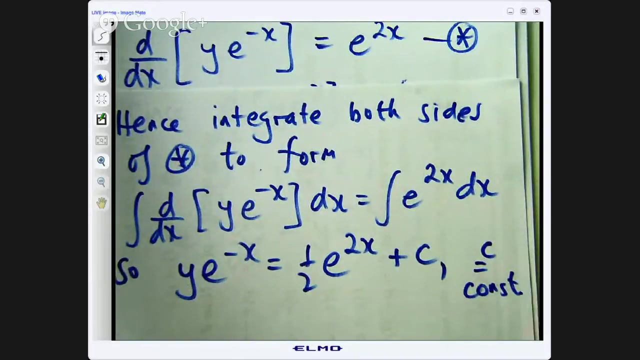 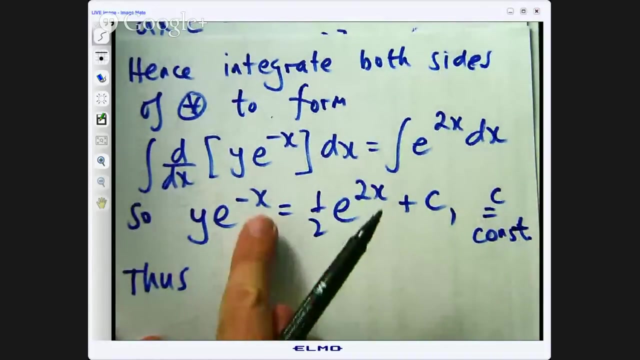 of integration in, So that is the integration on the left hand side, and I will put a constant of integration in, say c, where c equals a constant. alright, So now let us rearrange this and make y the subject. okay, Okay. Thus we are almost finished now. so let us divide both sides by e to the x, which is the. 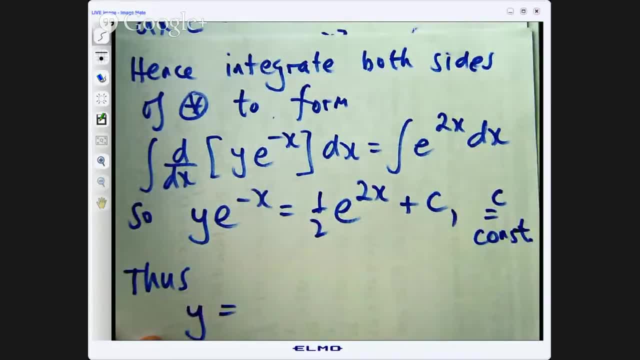 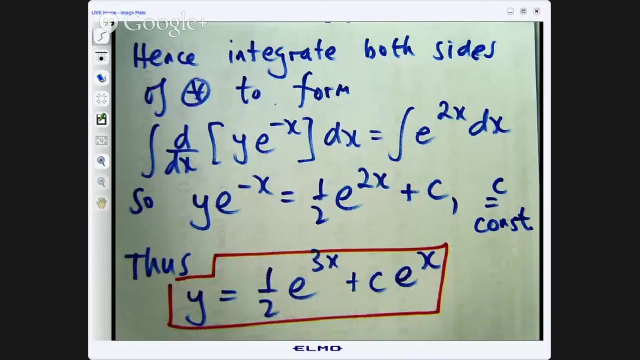 same as multiplying by e to the x, so I will get the following: So I multiply both sides by e to the x, I will get this plus c: e to the x. alright, So we have now spent a fair bit of time getting that general solution, okay. 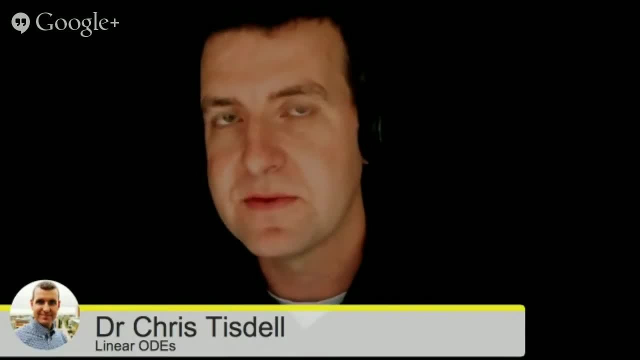 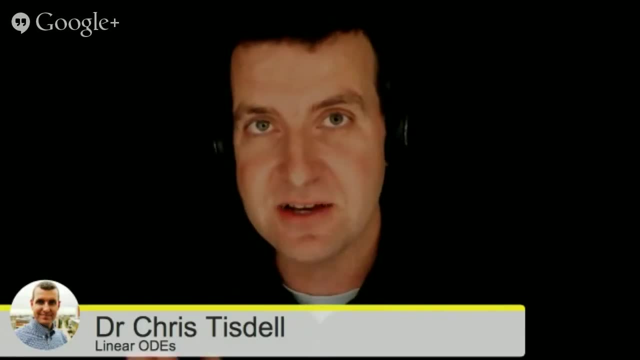 So with these kinds of linear problems, you are always going to find an integrating factor. multiply the left hand side- well, both sides- by that integrating factor and compress the left hand side down to the derivative of a special product involving the unknown function and the integrating factor. 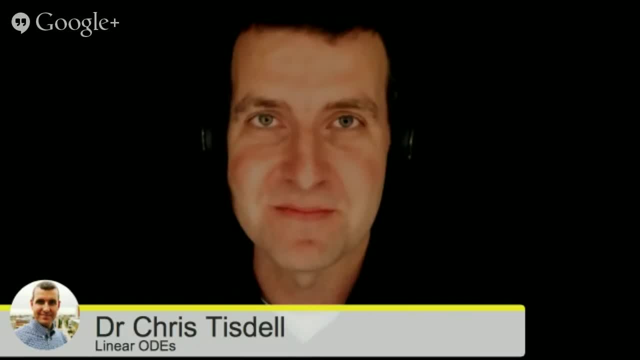 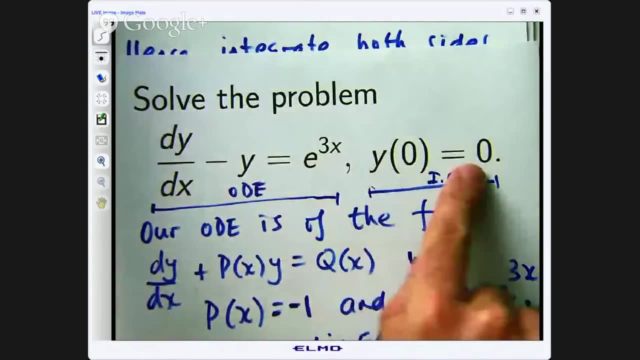 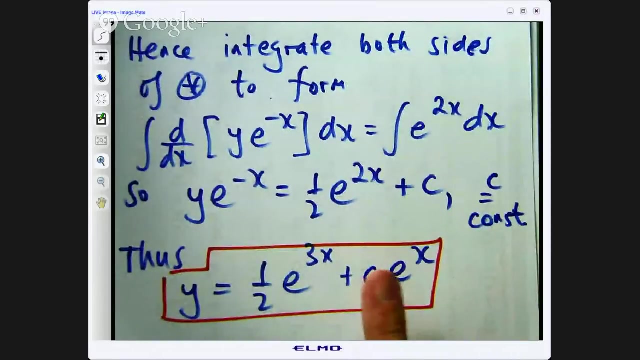 Alright, we are not quite done yet. What about that c in the general solution? alright, let us find that c. We have spent a lot of time using this equation, but we have not used this at all. So this initial condition is going to be used to refine the value of c in this general solution. 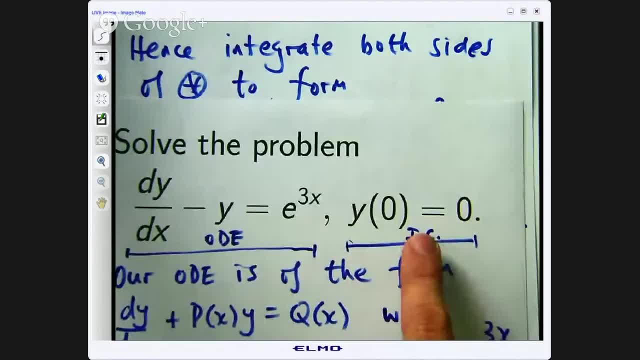 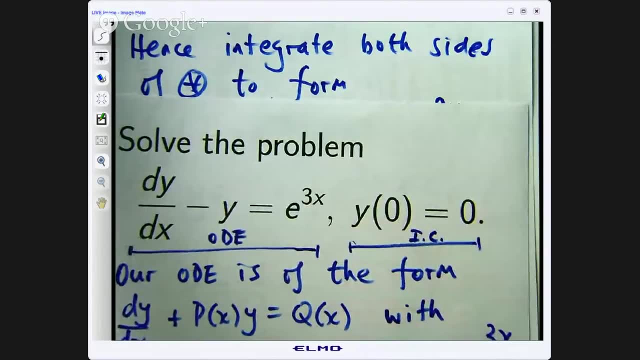 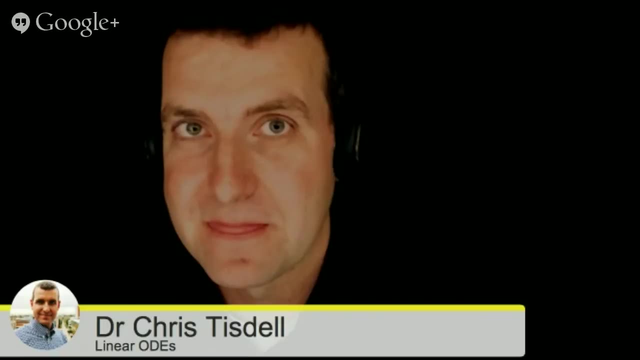 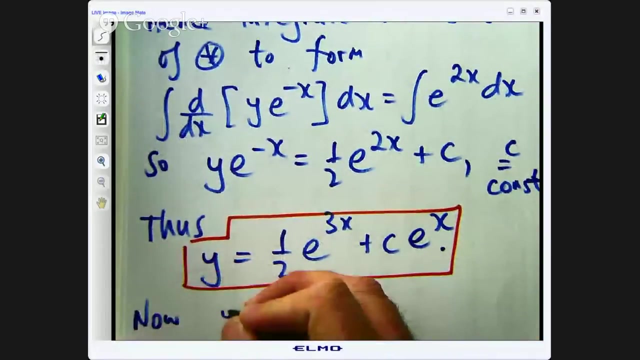 okay. So what this initial condition says is that when x equals 0, our function y should also equal 0. okay, Okay. So let us get a value for that c using the initial condition. Okay, this is known as a general solution. Now, y equals 0 gives the following: 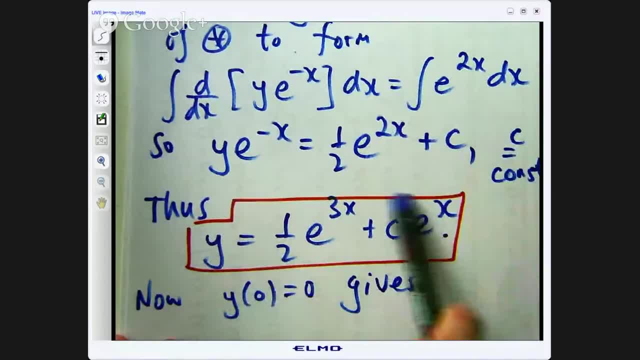 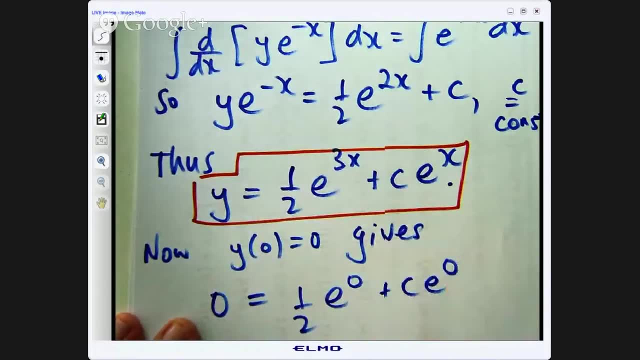 Okay, let us replace y with 0 and x with 0 in here. So e to the 0 plus c, e to the 0.. Okay, So e to the 0 is just 1.. So let us rearrange and make c the subject. 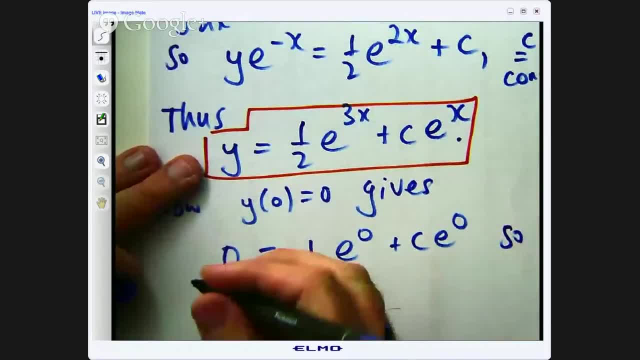 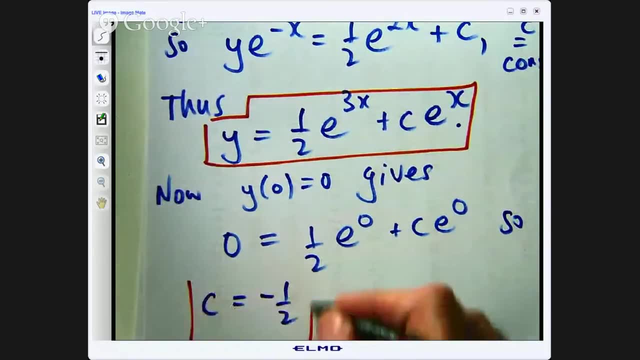 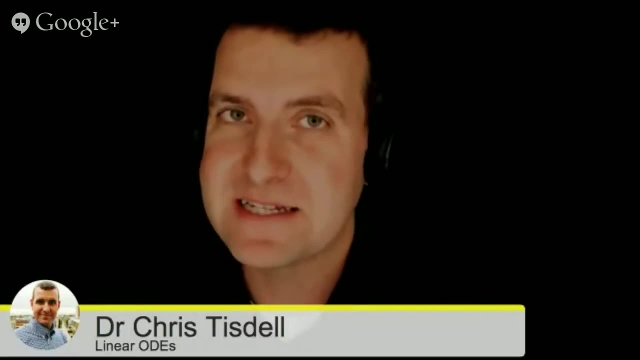 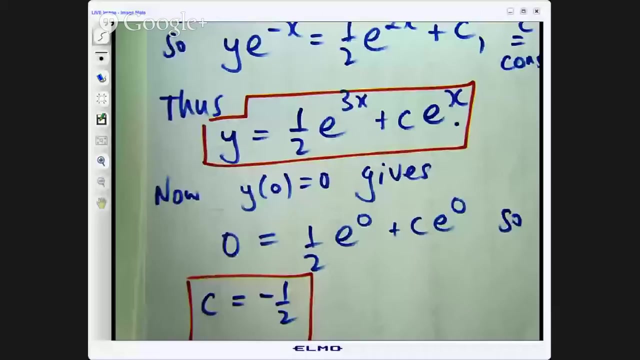 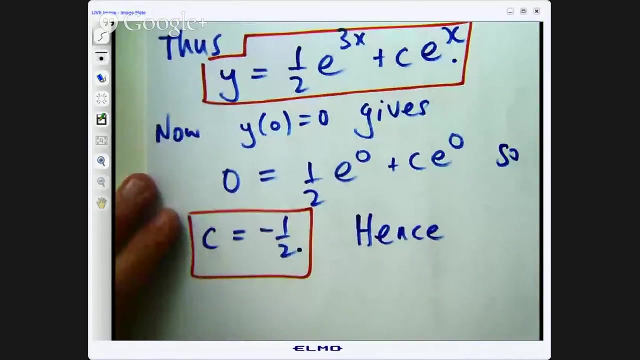 Okay, so that will go to the other side and I will get c equals negative one half. Okay, let us put it all together now. We are going to replace the c in our general solution with negative one half. Okay, so this is known as the general solution. 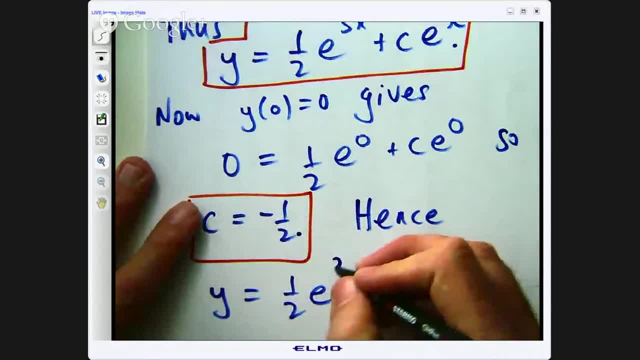 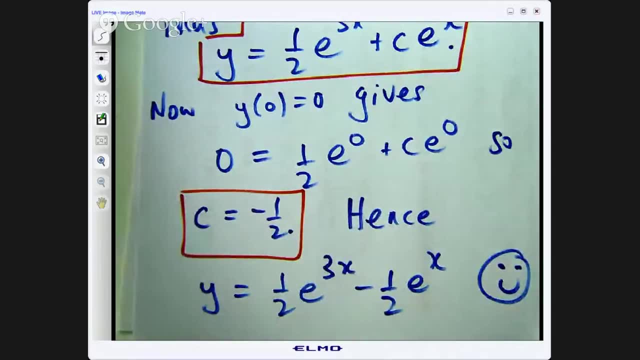 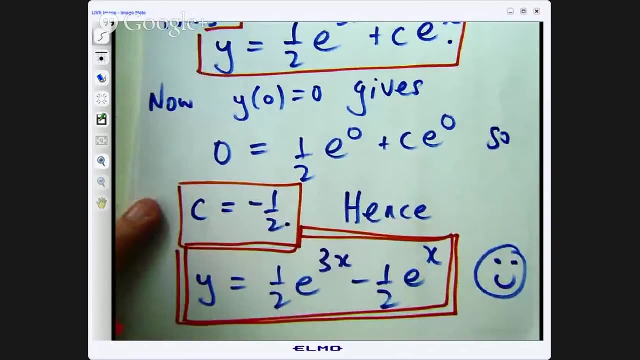 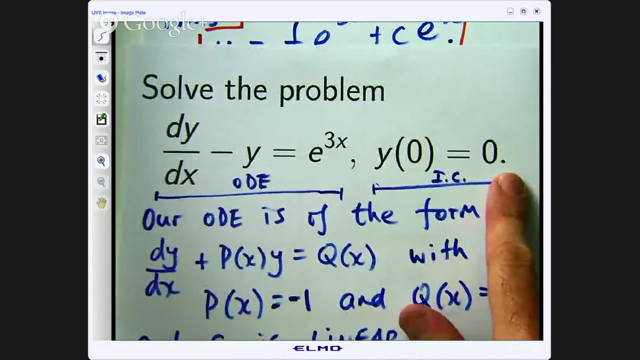 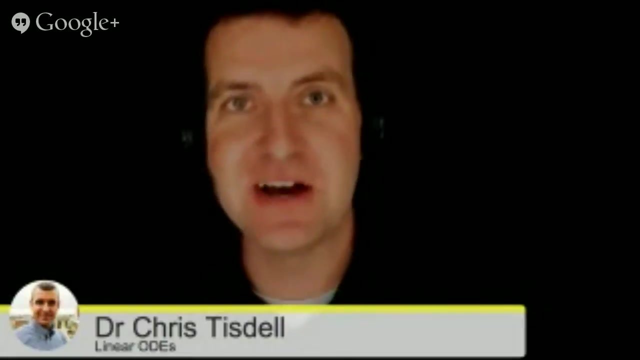 So we are going to replace the c in our general solution with negative one half. Okay. So negative one half, Okay. Hence, There is our solution to our original problem. it took us a while, but we got there. Now, how do I know that the function that I have come up with is actually the correct? 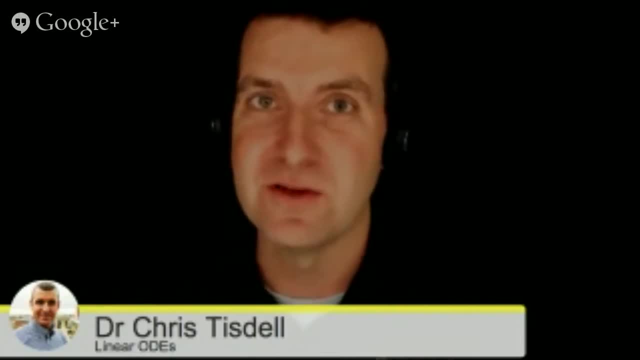 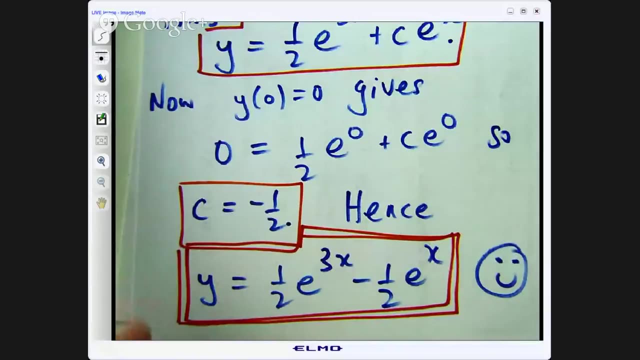 function. How do I know, How can I check that it is right? Well, I am glad you asked. let me show you. We can take this function and test it. We can calculate its derivative and then take the function y away from the derivative and 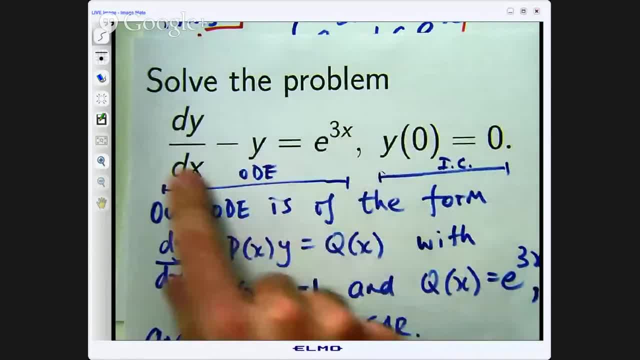 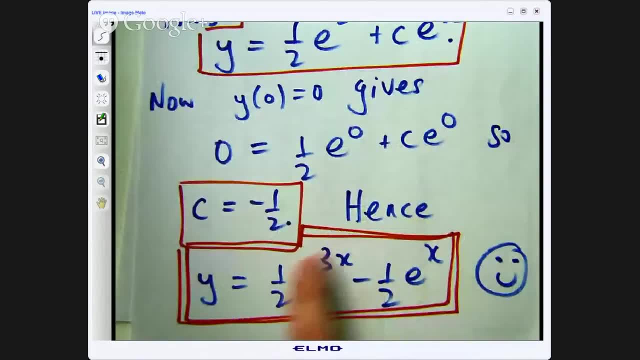 see if we get e to the 3x. If we do, then it definitely satisfies this problem. if we don't, then it is not a solution. We can also take x equals 0 and plug it in here. Do we get 0?? 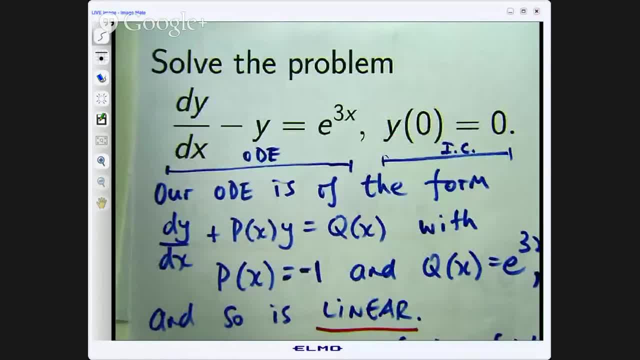 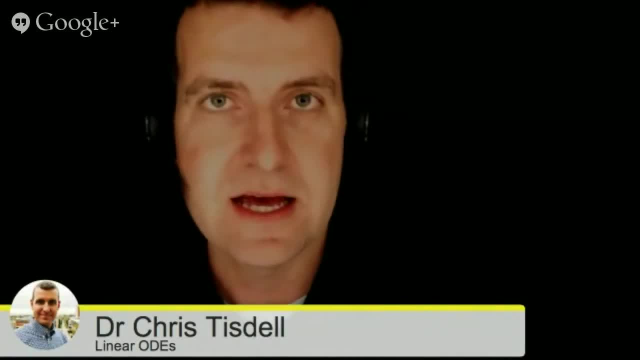 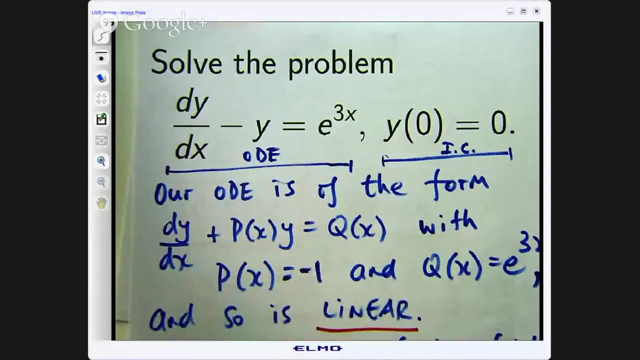 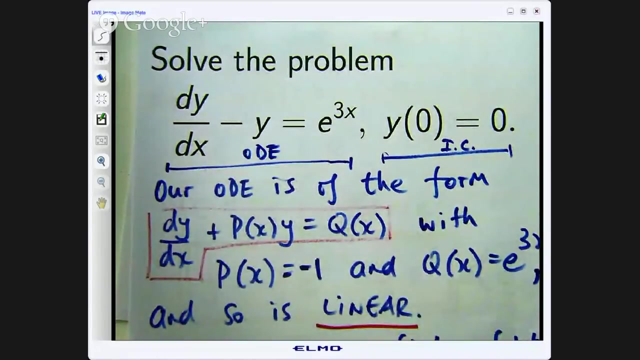 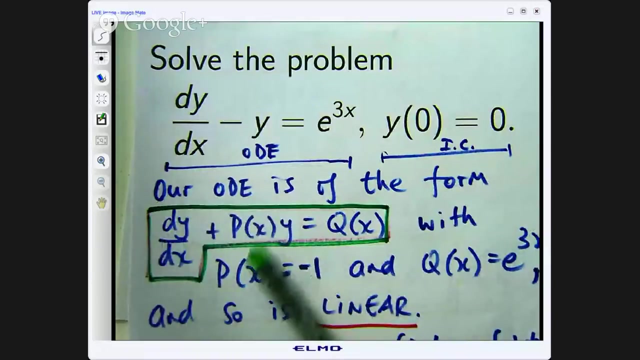 If you do that, you will see that this is satisfied and this is satisfied. Okay, so that is a linear ODE solved In fairly detailed form. let us just run through the arguments one more time. First of all, we identified that our ODE was of a special form. this form here and in this. 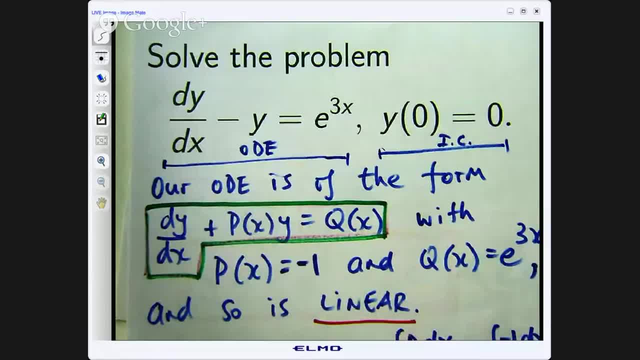 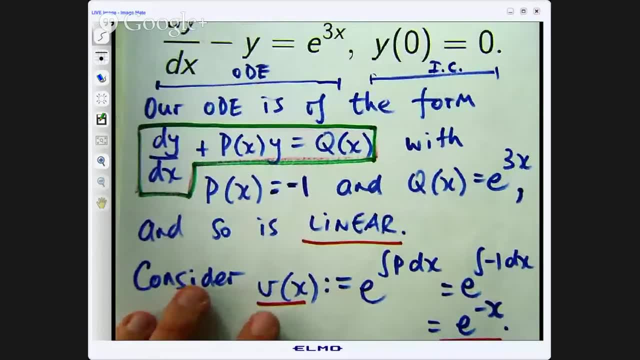 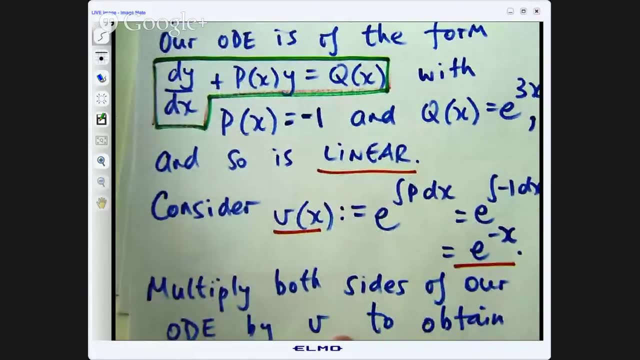 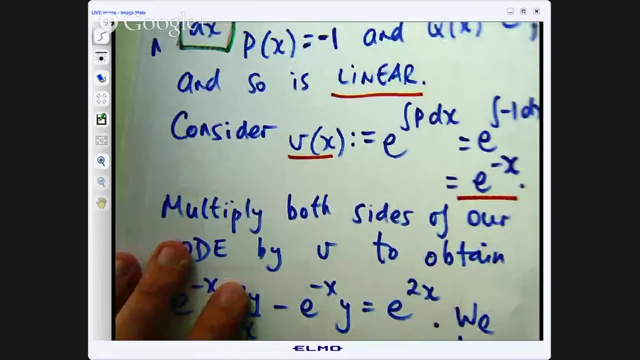 case p. Then we formed a magic function called an integrating factor from this p function e to the integral p. We then multiplied both sides of our ODE by this special function to form this and compressed this left hand side down to the derivative of a special product involving the unknown.